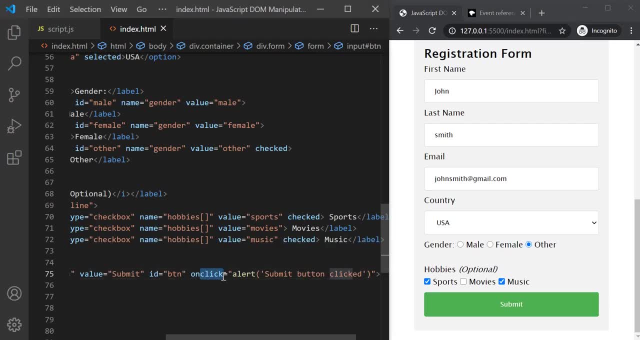 And the attribute name is event name prefixed with on. So if the event is click, we have to prefix it with on, So on click. If you want to handle focus event, then the attribute name should be on focus. If you want to handle mouse over event, then the attribute name should be on focus. 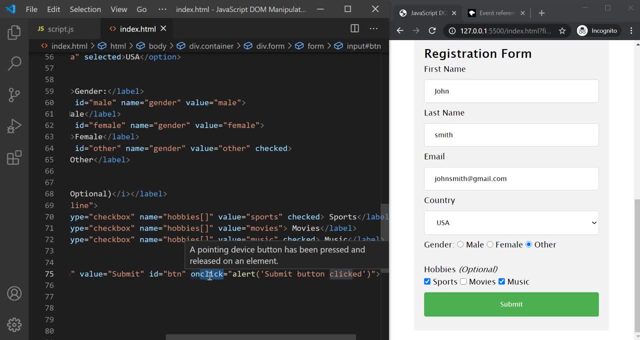 Attribute name should be on mouse over And to this we are assigning a JavaScript expression, And this JavaScript expression gets executed when that event happens And that's why, when we click on this Submit button, the click event will happen And it will execute this JavaScript expression which we have assigned to this on click. 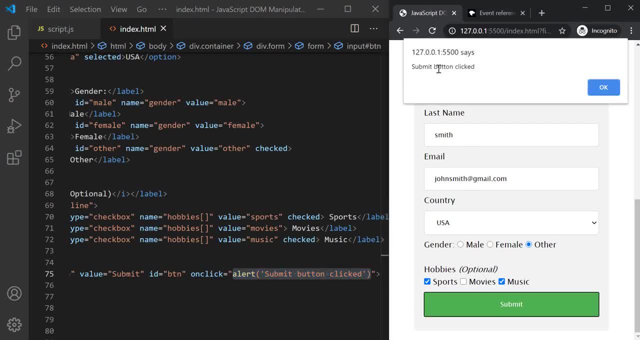 And that's why we see this alert window With this message Submit button clicked, And that's what we have specified for this alert. you know this alert function All right Now here. we are simply assigning a JavaScript expression here, But we can also do it something like this: 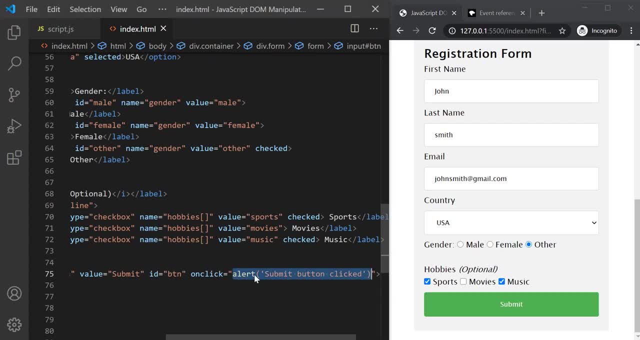 We can, you know, assign a JavaScript function to this. on click event. On click attribute. So let's say we, when this click event happens, we want to execute a function, And let's say the function name is display alert. Okay, so we want to execute this function. 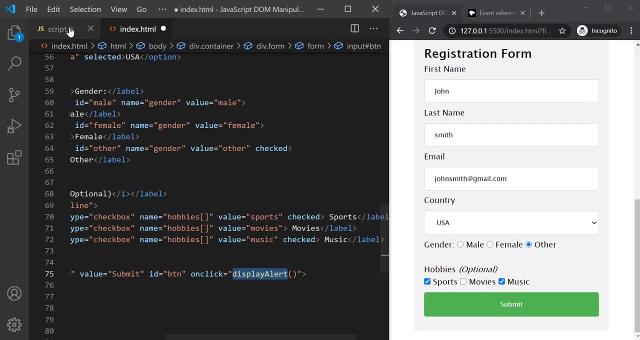 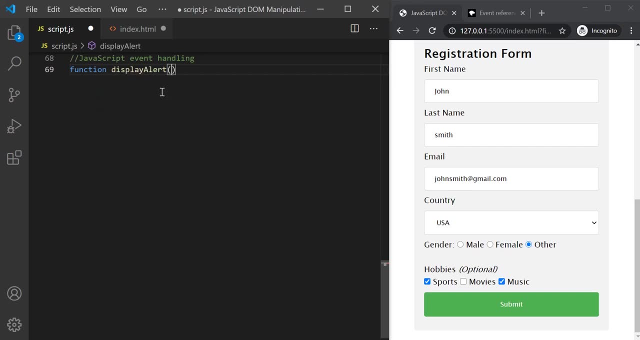 Now we don't have this function in our JavaScript code, So let's create this function, So let's use this function, So let's use this function- keyword, And then the function name, And inside this function, let's write the logic which we want to execute when the click event happens. 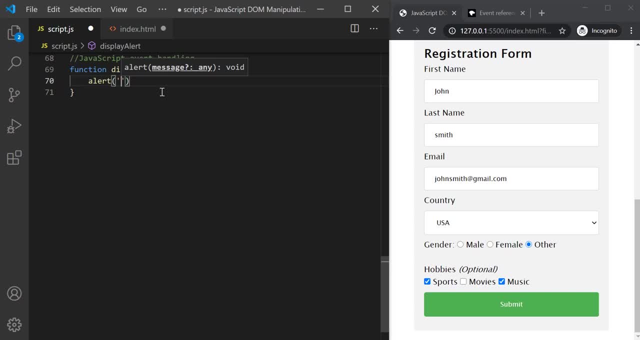 So here we want to execute the, we want to display this alert window. So let's say: Submit button clicked, Let's save the changes And again, when I click on this Submit button, it should display this alert window With this message: Submit button clicked. 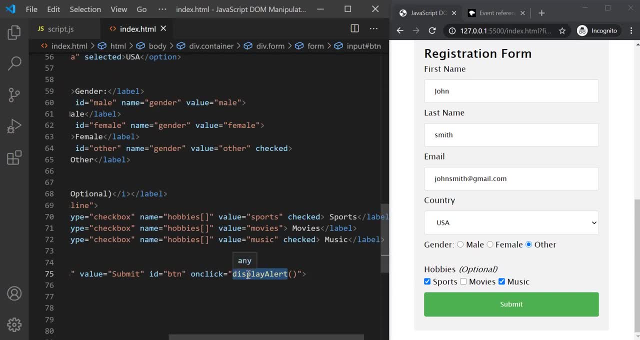 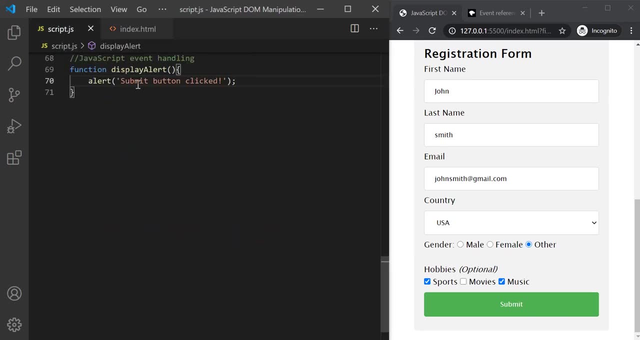 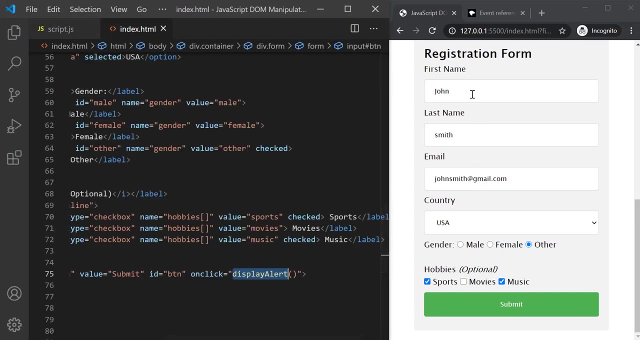 So now, instead of executing a JavaScript expression here, we are calling a function And whatever code we have written inside that function, that will get executed when the click event happens. Let's see another example. So let's say, when we click inside this first name text box, then we want to change its background color to yellow. 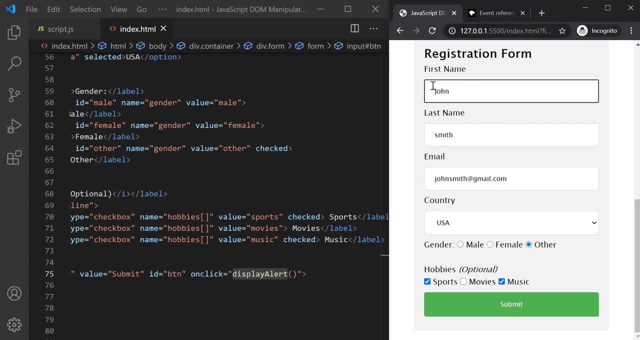 Now, when we click inside a text box Inside a text box, the focus event happens. So here we want to handle the focus event for this first name text box, So let's scroll up to the element for this first name text box. 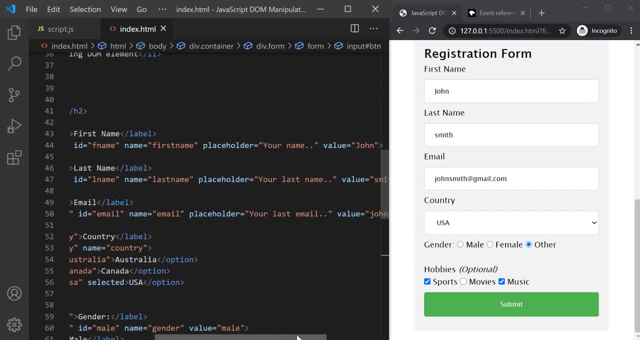 And here it is. And to this, let's create an event handler attribute here And what should be the name of the event handler attribute? Since we want to handle focus event, the event name should be- I mean, the attribute name should be- OnFocus. 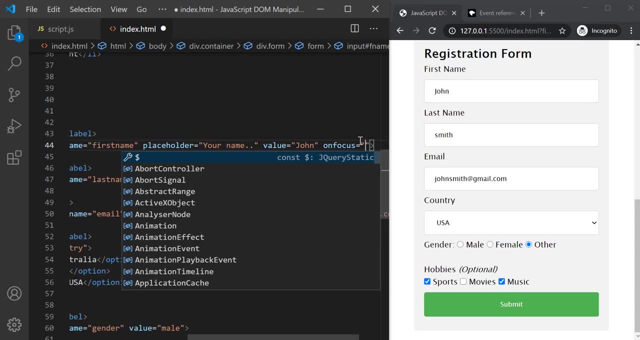 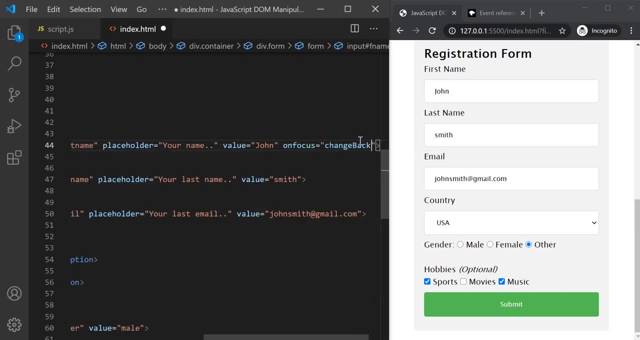 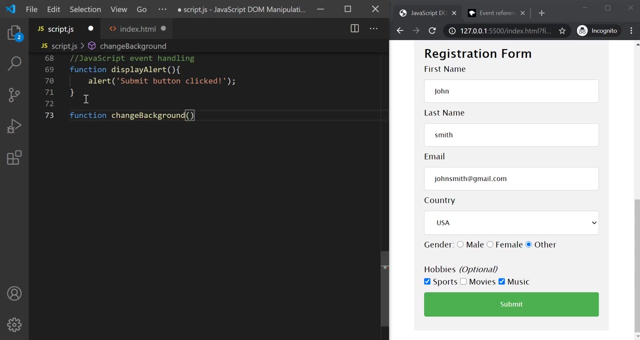 And to this OnFocus Let's assign a function which will get executed when this focus event happens, And let's call this function: maybe change background, Okay, And in the JavaScript code let's create this function. So function: change background. 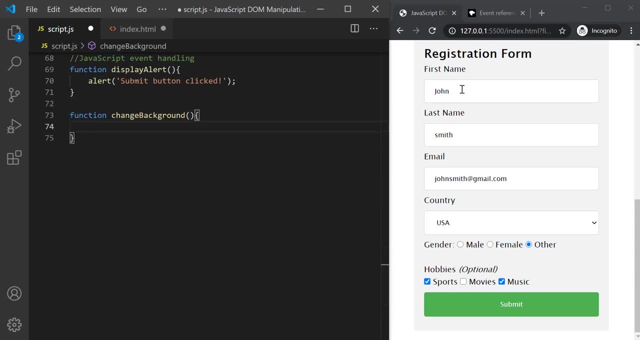 And here we want to change the background color of this text box when OnFocus event happens. Okay, So let's say, let's first get access to this element. So documentgetElementById and id of this element is fname, I guess, Okay? 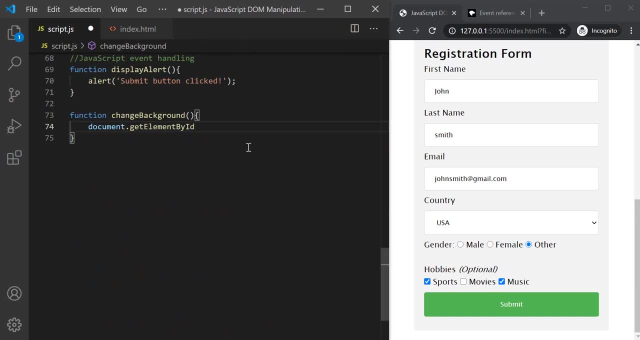 It is fname, So let's use this id. Okay, And let's pass this to getElementById method. And let's say dot, And we want to change the background color, So for that first we will have to use the style property. 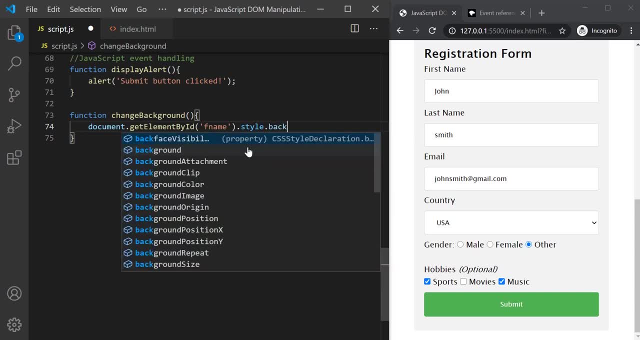 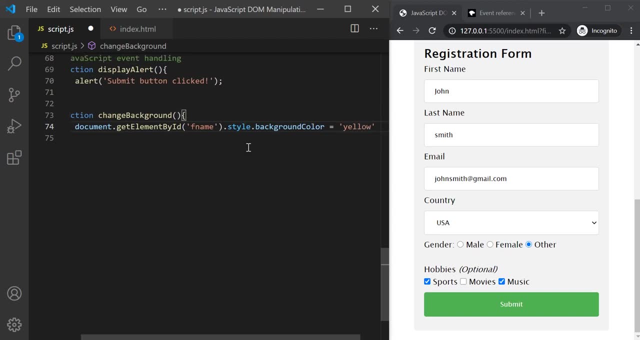 On that style property. we want to use the background color- You know Property- And we want to set it to yellow, So yellow. If I save the changes now and when I click inside this text box, the OnFocus event happens. 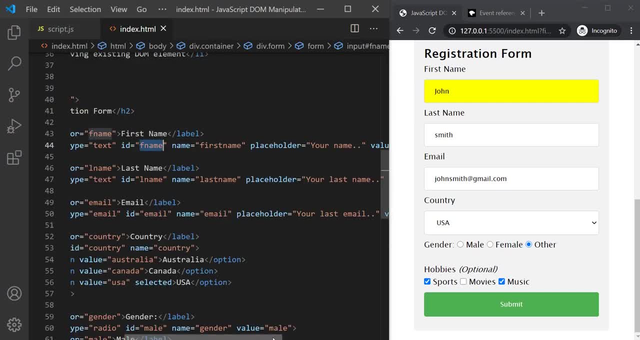 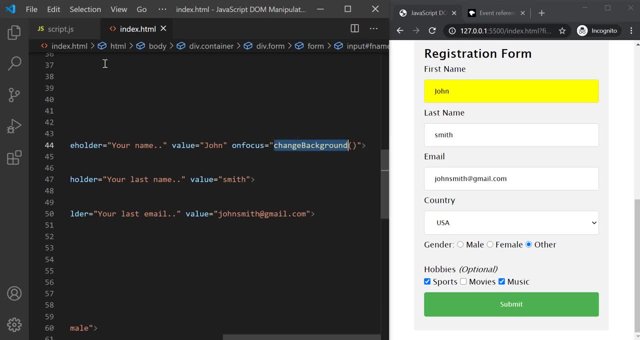 And when OnFocus event happens, this method which we have specified for this OnFocus attribute, this JavaScript function gets executed. Okay, And inside this JavaScript function, we are simply changing the background color, And that's what you see here. So in this way, you can add event handler attributes to the element which should listen to an event.